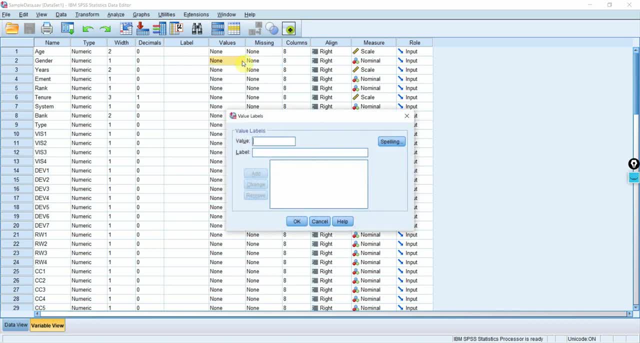 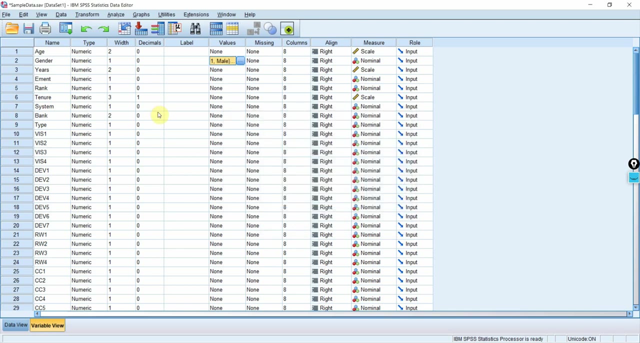 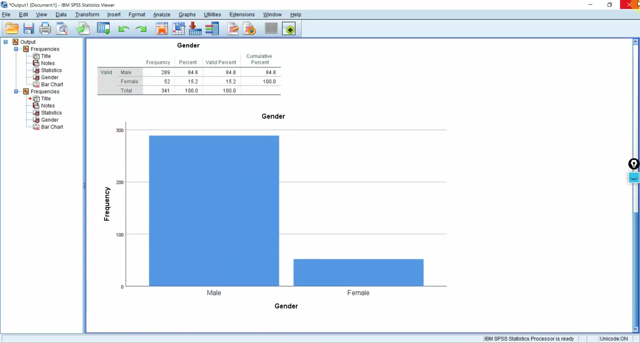 In the gender for the values. select one male, two castle female, Press- okay. Now let's do that again. Analyze frequencies, Press- okay, And here are your results: male and female. Now there are many other types of plots and charts that can be done, So for that we've got a specialized menu. 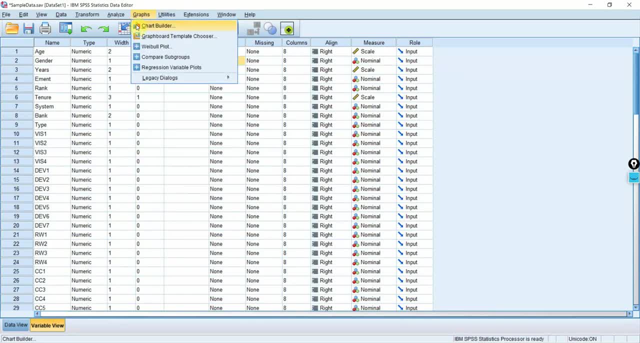 here, graphs, chart builder. We can use chart builder in SPSS because by colouring them, the chart will display a variety of different SPSS to build our own charts. so let's- and there is legacy dialog, and it gives you all these charts. 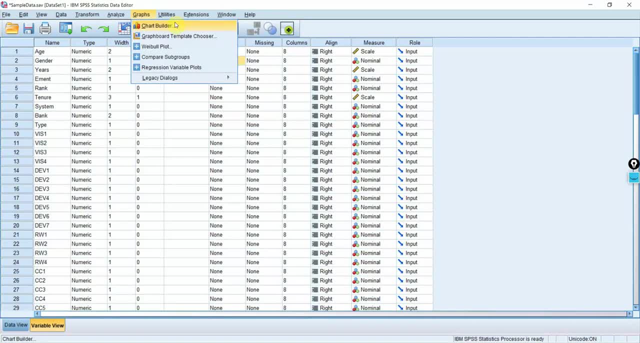 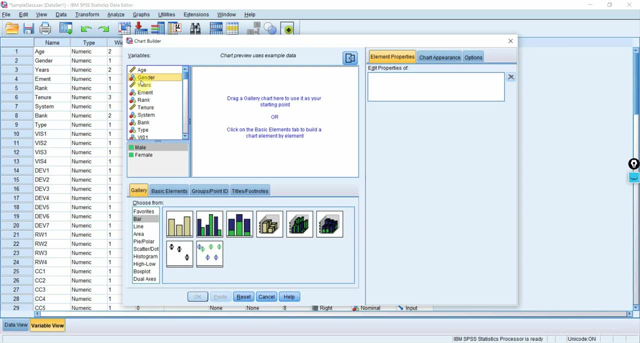 separately as well. so let's use chart builder for now. so click chart builder now I want gender. so what I'm going to do is, let's say I want bar chart, simply drag it and drop it onto this chart here. now I want bar chart. select your bar chart, double click on it and I want. 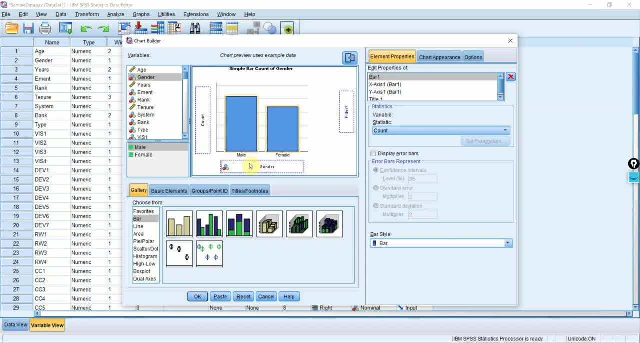 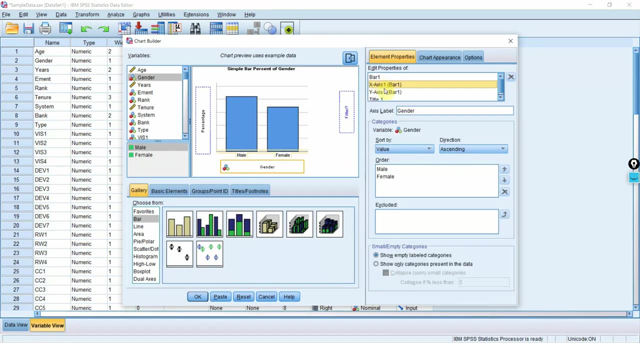 gender. here I've got just one single variable. that's about it, nothing else, and the statistics that I want. you can have percentage as well. nothing else needs to be done. your x-axis, y-axis, but in this case it's just a single variable. you can have chart appearance as well. you can play around with these. 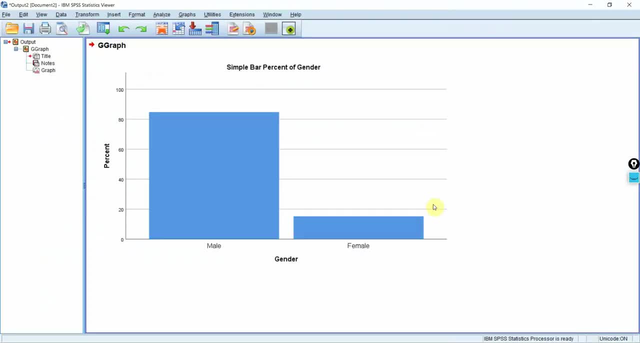 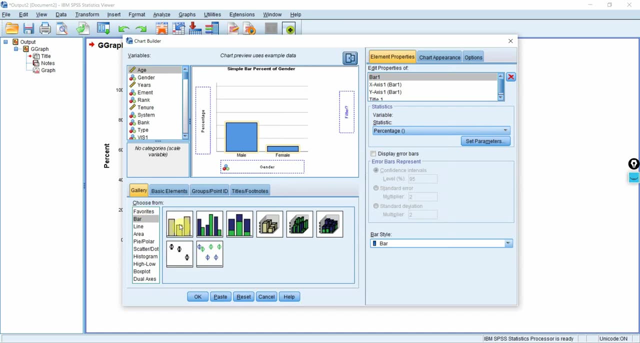 and just press ok. now here are your results. now let's do another one graph chart builder. let's say I want pie chart, so I'm going to click here, drag and drop it here and again. gender is already selected. that's it. now let's press ok. 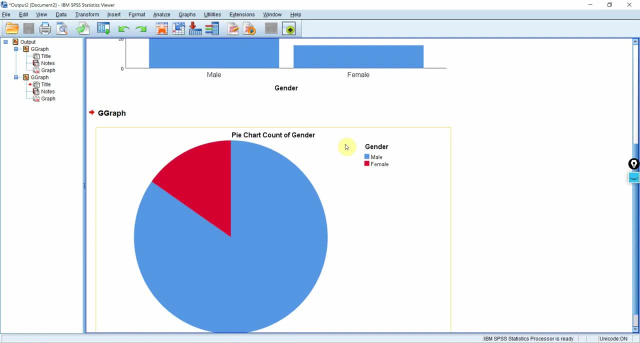 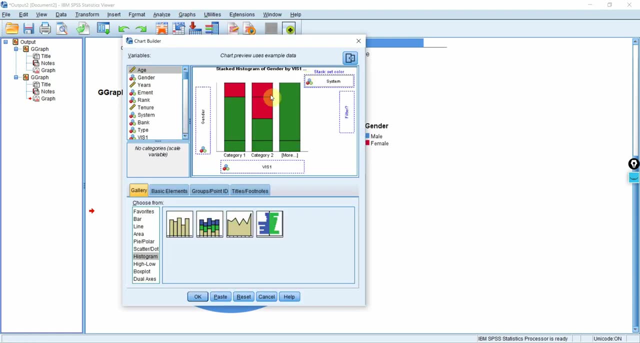 and here is your pie chart for gender. moving on, let's try some other graphs as well. now, if you want to clear the canvas, just right click here. now it is clear. now let's add histogram. let's try a simple histogram for this variable here: vision, which is one of the variable. now you 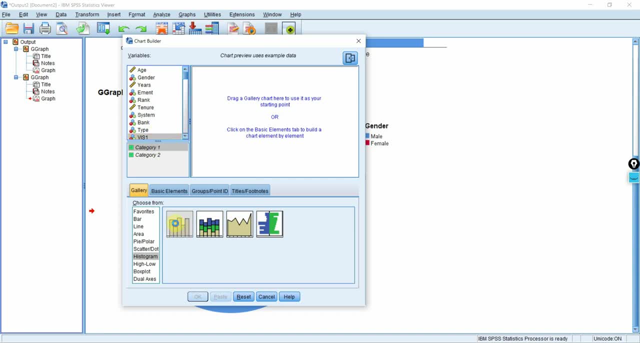 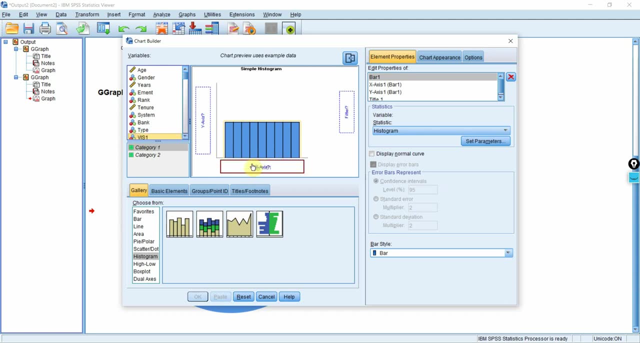 cannot add it. before you add it, you can hit hit to add a graph, so just please double click on it once it is added. now add your histogram or the variable that you want to assess using histogram. just put it in here and let's press ok and this is your. 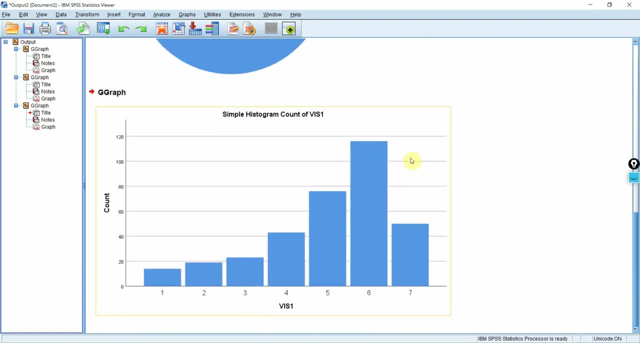 histogram. well, it is not normally distributed because the values are more or less showing a tendency towards the right side of the graph, that is, higher values now. similarly, you can have legacy dialogues and let's say: i want a bar chart. you can have different bar charts. let's say i want a simple one: press define. 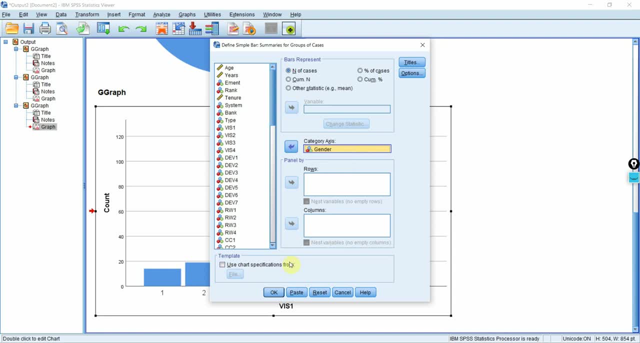 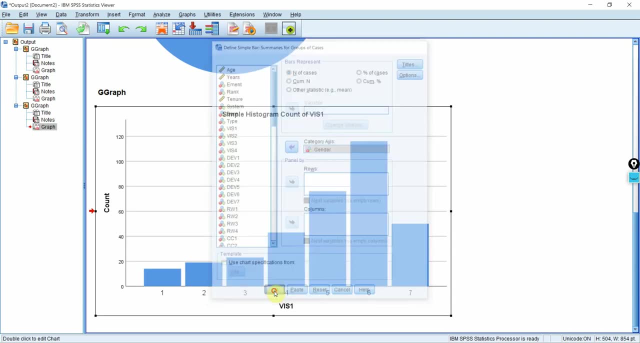 so let's say i want it for gender, that's it, nothing else you can have. or you can define the panel by rows and columns. we are just going to look into it. that, as well as to what we get, press ok, and the same bar chart that we got earlier. now let's change it a bit. go to graphs. 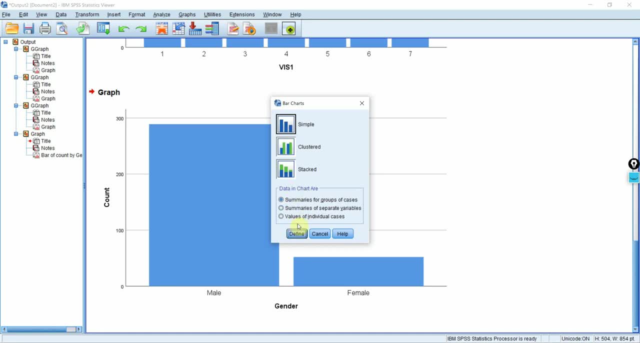 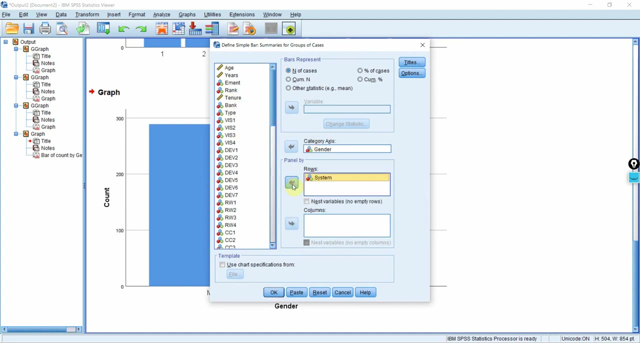 legacy dialogues. use the simple one: summarize for groups of cases, summarize for separate variables, summarize for individual cases. now, in this case we are going to- we are just going to use group of cases, define and, let's say, i want to look into system, just press it as system here. 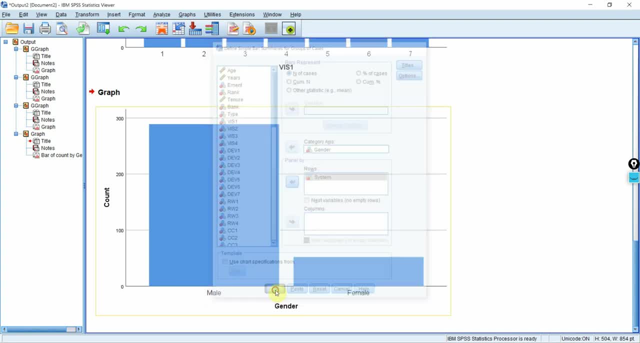 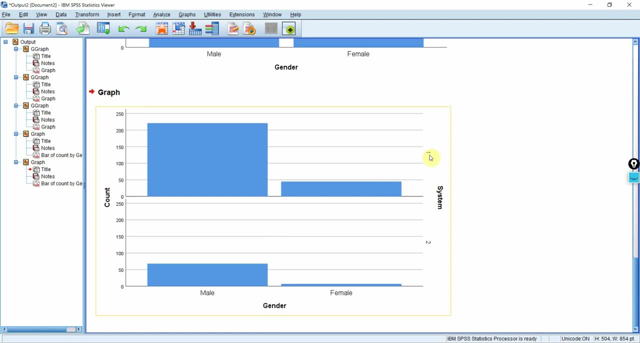 let's use the number of cases. you can try different options and see how the output changes. now this is system number one, that is, private sector banks. this is in system number two, public sector banks, and in public sectors banks. this was the number of male respondents and female. 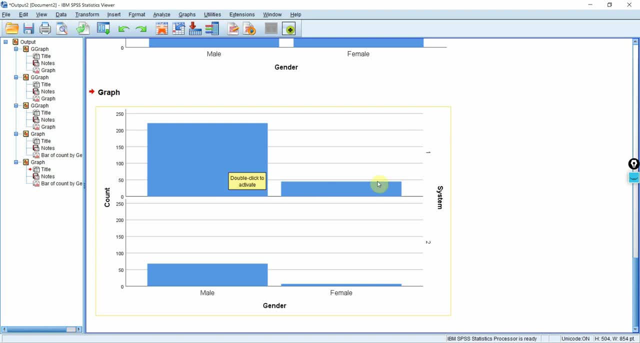 respondents, and this is for private sector banks. so you can divide your graph into different categories based on a certain variable as such, well, following, you can have different plots as well. you can have scatter plot, for example. you are testing and the regression assumptions, so let's choose a.